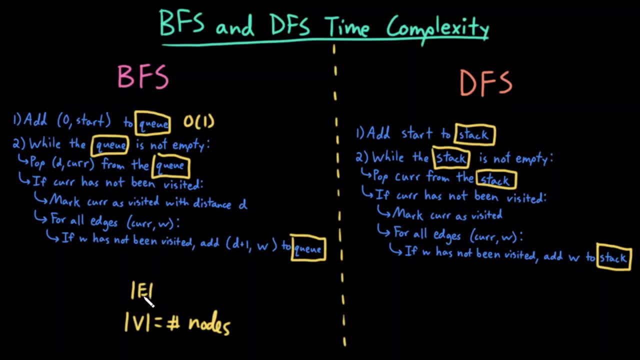 of the nodes on a set of nodes and by adding a parameter to the set of nodes we get the set of is the number of edges for both examples, not just for BFS. Okay, so in the worst case, popping off one element from a queue. well, a queue is always constant time I can add or remove. 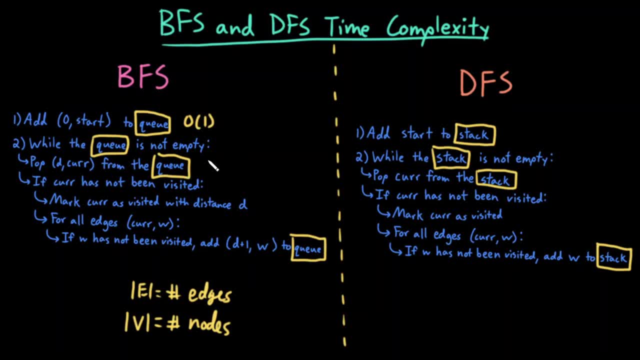 to the front or the back in constant time if I implement my queue using a linked list, So this is just constant time. If the current node has not been visited, that check is constant time. I just look up a Boolean mark it as visited, So that's just. 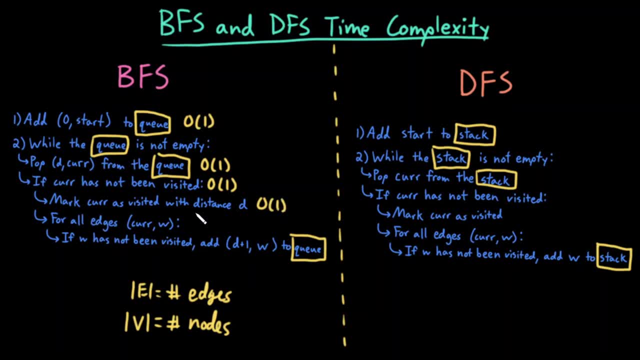 an assignment That's constant time for each of its outgoing edges. Well, I could theoretically have a network where my current node has all of the edges in my graph as its outgoing edges. So, technically speaking, this step might have to iterate over every single edge in my graph If the current node, if the neighbor, has not been 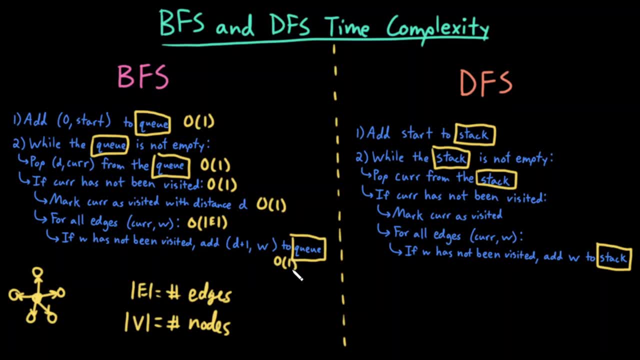 visited, potentially added to the queue. this is also constant time. So we have this big O of E term And theoretically we might have to iterate over the queue, big O of E times, But the overall time complexity, despite what you might naively think, it's not actually big O of E squared. 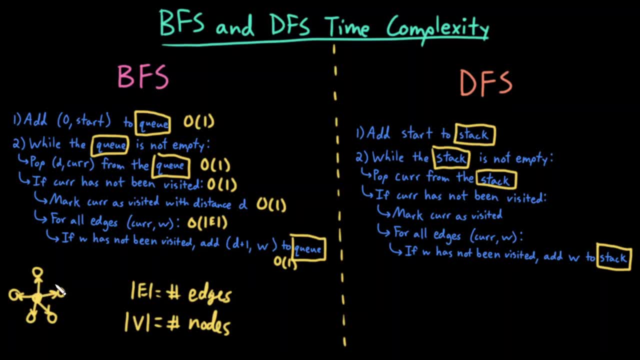 Note that, no matter what the structure of my graph is, so regardless of if I have all of my edges coming out of one node, or all of my edges or all my nodes having exactly one edge, regardless of the structure, I only add each edge to my queue exactly once, So I only operate on every single. 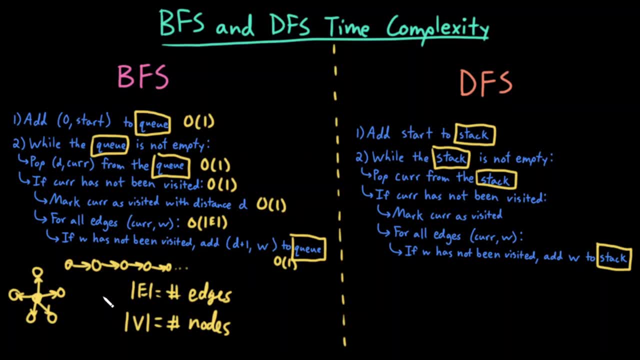 edge exactly once. So in reality, this entire while loop, including all of its contents, is just big O of E. I might have to do some constant time operation for each of my big O of E elements. In reality there's usually. 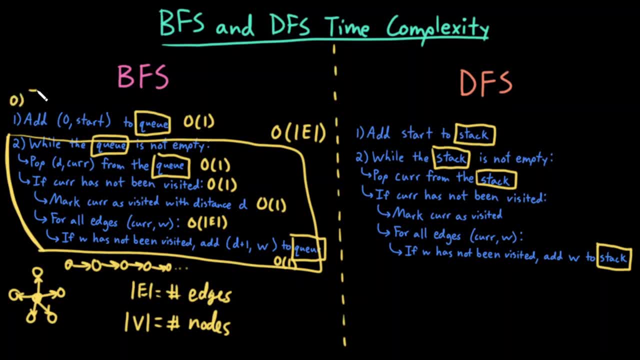 a first step before I even do my breadth-first search, which is initialize. So, for example, if I want to find the shortest path between my start node and any other vertex, I might have to initialize some previous pointer, for example to keep track of what node was. 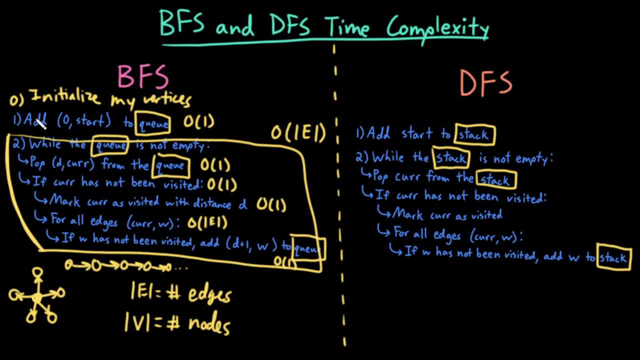 the one before me. In general, I might have to initialize something for each of my vertices which would be big O of V. So, generally speaking, if I include any graph initialization and I have my BFS traversal, the overall algorithm of BFS is big O of V for the initialization. 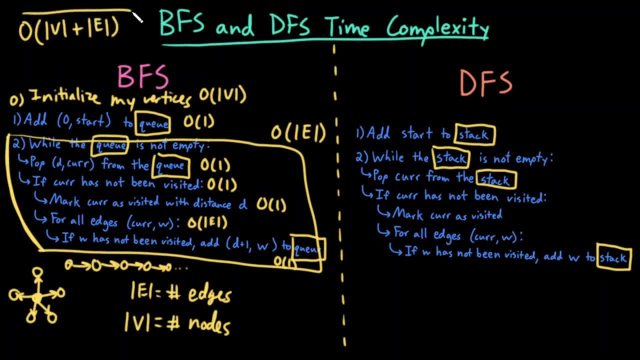 plus E for the actual graph traversal the actual BFS. Similarly for DFS, I would probably have some initialize the vertices step. So initialize all my nodes- This says vertices here- And notice that the algorithm is identical, except, instead of using a queue, I'm using 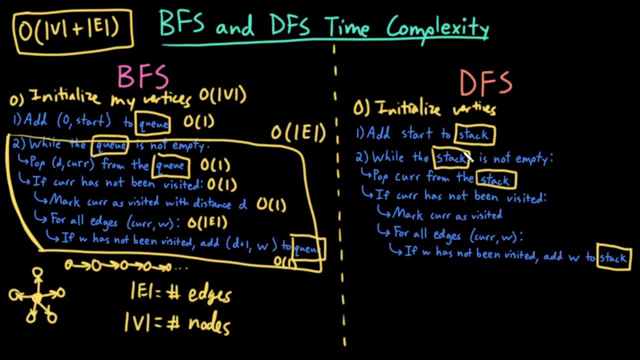 a stack. Well, remember, if I use a linked list to implement my queue versus a linked list to implement my stack, in both scenarios I have constant time access to the front or the back, which means that I have the exact same time complexity as BFS. It's actually. 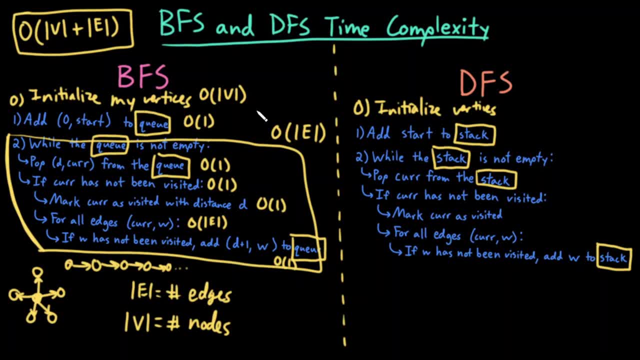 the exact same algorithm, except I have constant time access to the front or the back, which means that I'm changing the order in which I'm iterating over my nodes And, as a result, the paths that I traverse look different. So, because it's the exact same algorithm with 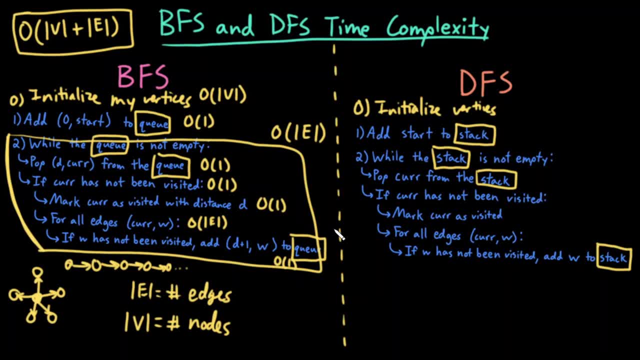 the exception of swapping out the data structure, but the data structure has the exact same Morsky's time complexity. DFS is also big O of V to initialize my vertices plus E, because I have to theoretically do a constant time Operation for each of my big O of E edges.